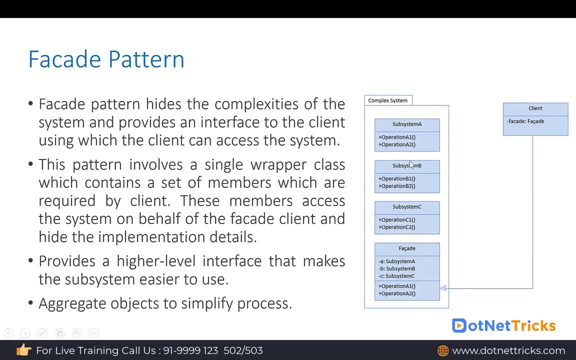 performing so many operations over there. So, instead of exposing all these operations, what we will do? we will create a facade wrapper. In the facade wrapper, we are calling the subsystem 1, subsystem 2, subsystem 3.. We are calling the subsystem 1, subsystem 2, subsystem 3.. 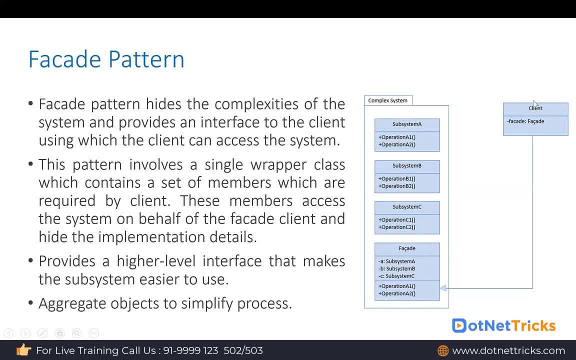 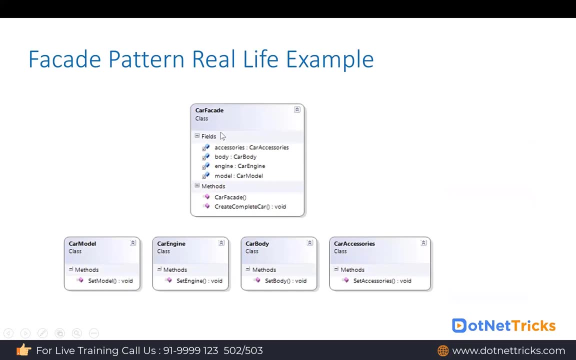 This facade objects will be exposed to the client Instead of exposing these subsystem where internally, when it is coming to the the car manufacturing process, in the car manufacturing we So let's say we have in the car model where we are setting the model, information engine. 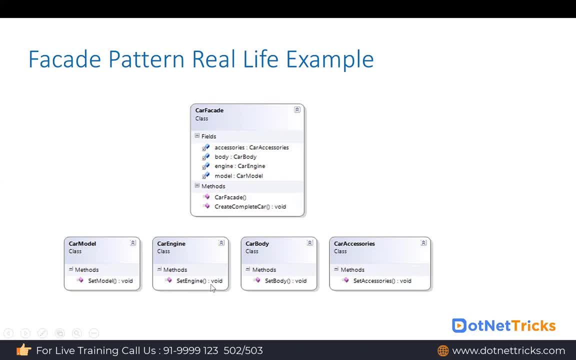 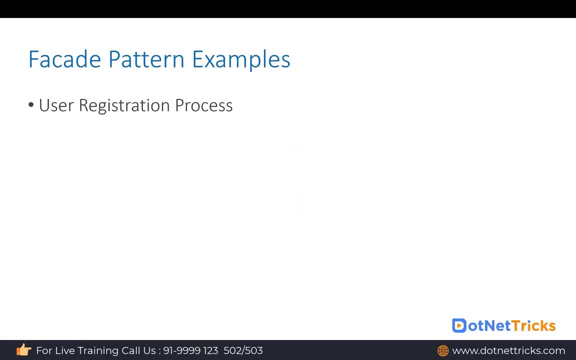 let's say body car accessories. so it's a complex one. There can be another example. let's say we are having a user session process and in the user session process, behind the scene, you might be doing so many things. You uploading a picture over there, you are providing the permission to the user and 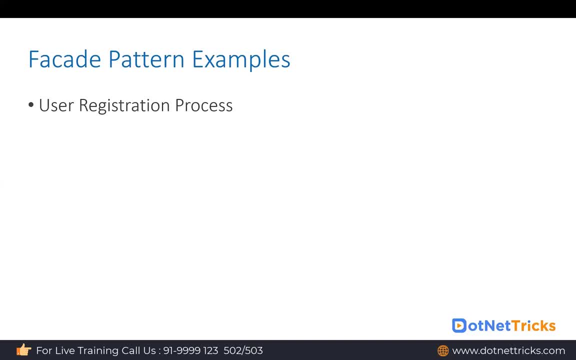 you might be doing some other operation, So the end user is not aware of what is happening behind the scene in the system. that is a complex process. The other example can be here: processing an order. So if you're looking at the Amazon, let's say the Flipkart, when they receive the order, 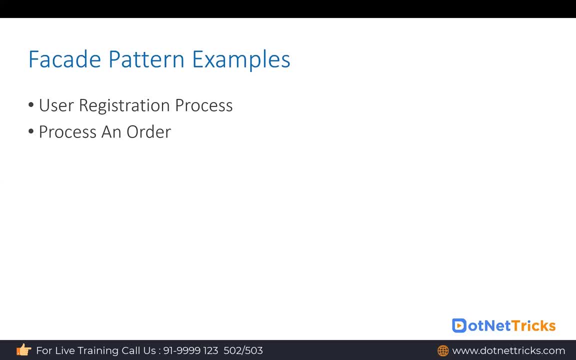 they do so many things behind the scene. They generate the invoice, they send the received order information to the vendor as well. Then vendor at his end start preparing the order. Then vendor provide the information about whether the order is going to ship or not. 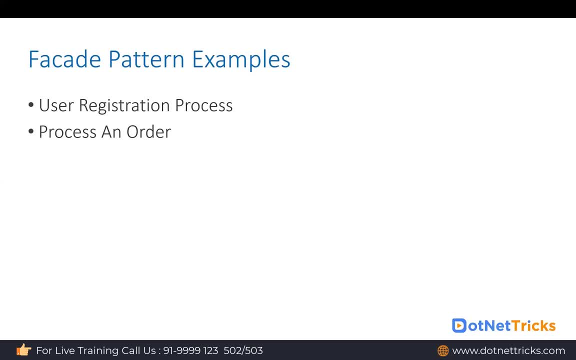 when it is going to be delivered. so it's a complete process behind the scene. a system is having, So it is also. the example can be simplified with the alpha facade pattern. There can be another example. let's say we are having a user follower. if you're looking. 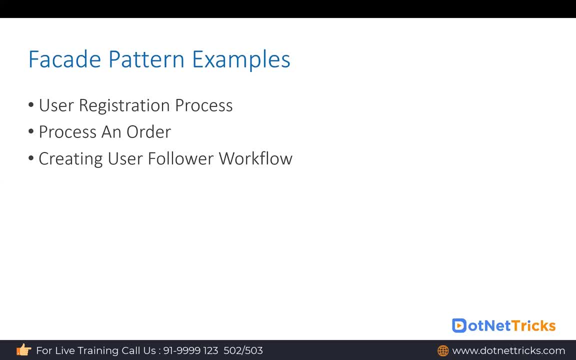 at when you follow somebody at Facebook. Okay, If you follow someone to it, let's say in Twitter, so to which person you're following, that person get the notification like this: is the person now start following to you. Even what are the your friends are having. your friends also can see like to how many. 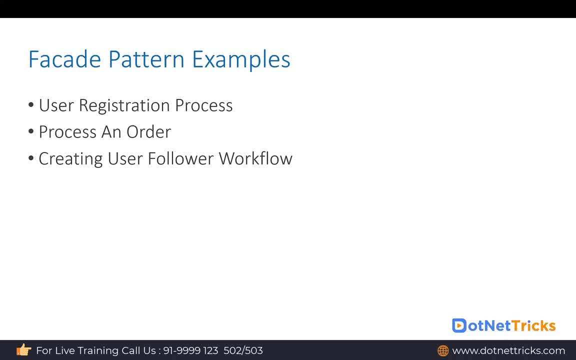 people you are following. So this is also a complex process behind the scene. It is looking like simple, Let's say I just need to click on a follow button, Okay, But after clicking on that follow button, behind the scene you have to do so many things. 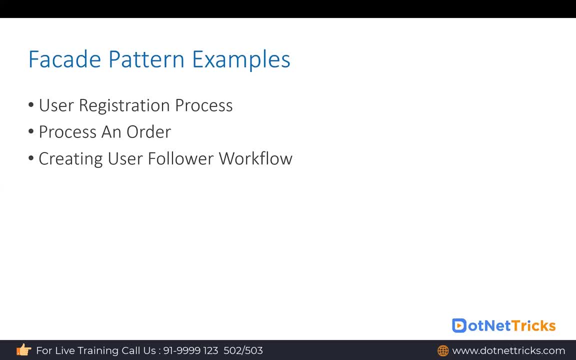 So this is also the example through the facade pattern you have simplified. So just create a wrapper class to follow the user, wherein to pass the user name and you need to pass the user to follow or internally. you have been so many process over there. 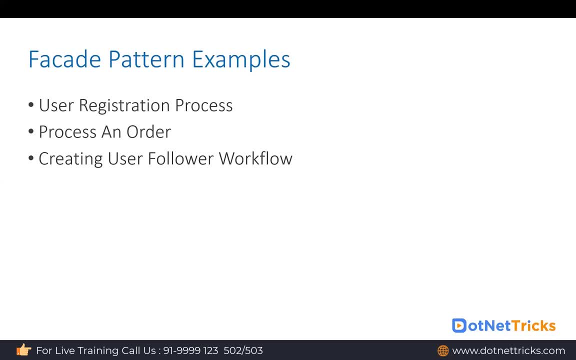 where you are storing the information to database, where you are sending the notification to the users. So if you follow someone to your home, you are following. then there can be another notification to your friends. They also get notified. Let's see, you started falling to someone else. 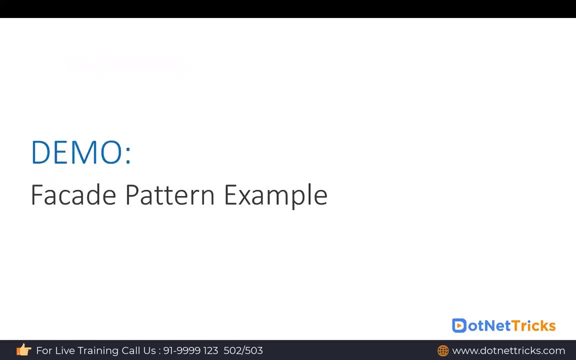 So these are some facade pattern example. for the facade pattern example, I'm taking the example of, let's say, how to follow a user. So let's say you are having a website. on the website You are having the option where the user having their own public profile similar to the Facebook. 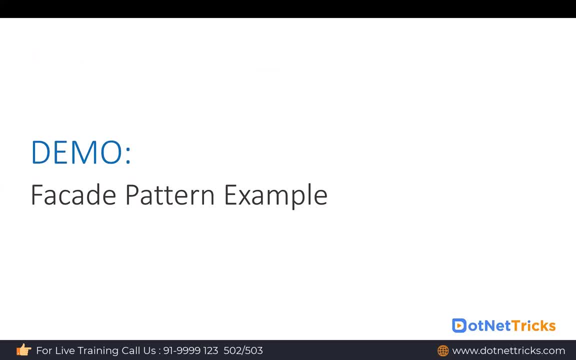 similar to the LinkedIn: Yeah, Somebody is going to follow you. Okay, Okay, a person, so that person will notified and if the follow process has been done successfully, I will also get the message. now you are falling to that person. even your friend also get notified. 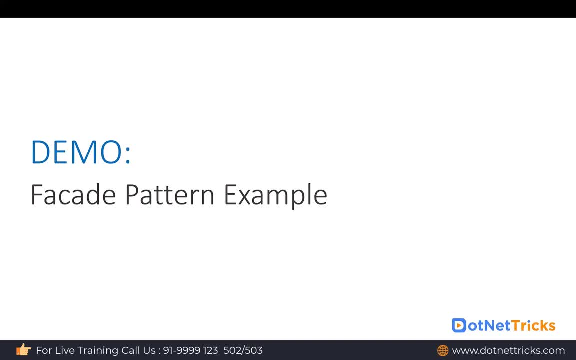 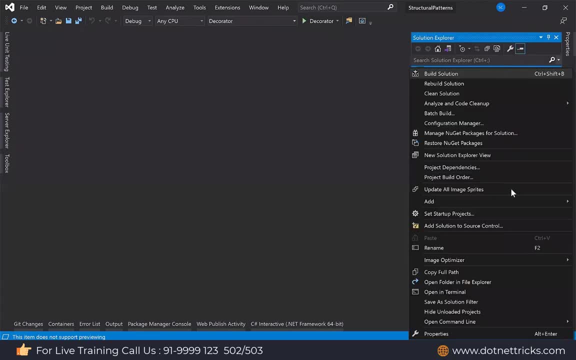 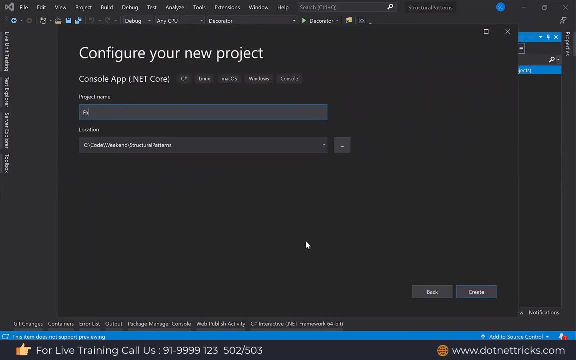 and now the person ABCD start falling to person XYZ this way. so let's see how the facade pattern can be implemented for this complex process. so what I'm doing here? I'm just adding a one more project, and the project name is here facade. so the same example I'm taking. 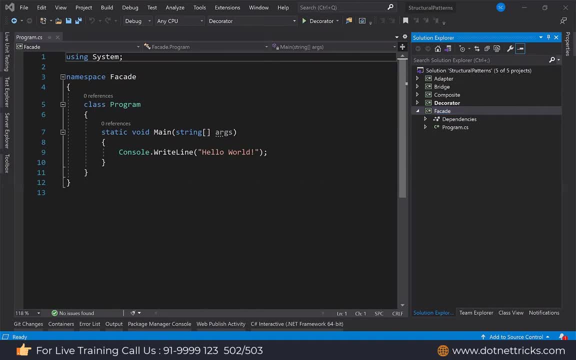 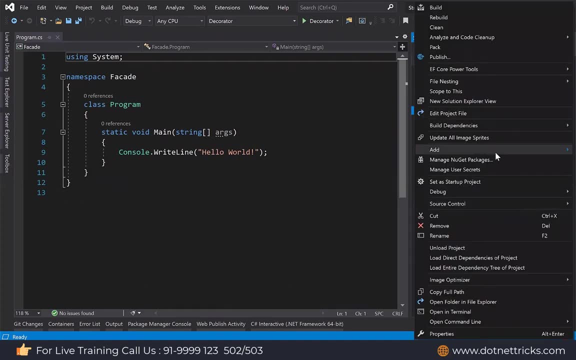 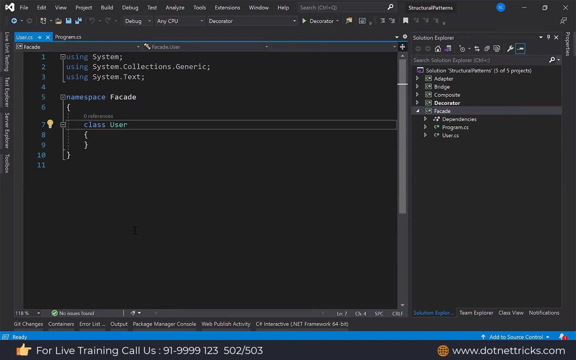 here where we are just going to follow to a user. so what we'll have here? we will have a user class. so I'm just going to create a user class- so public, public class user, where the code we will define and we will have a class for the follower. 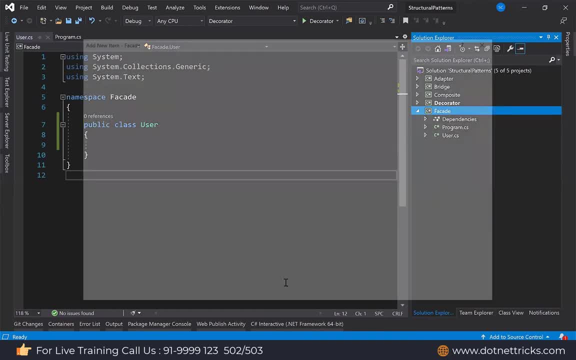 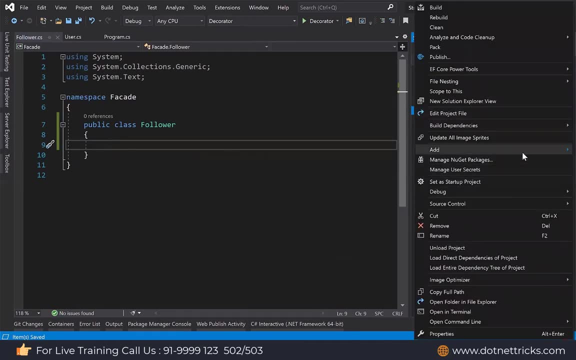 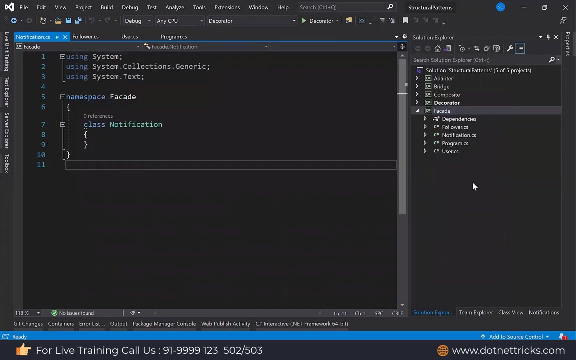 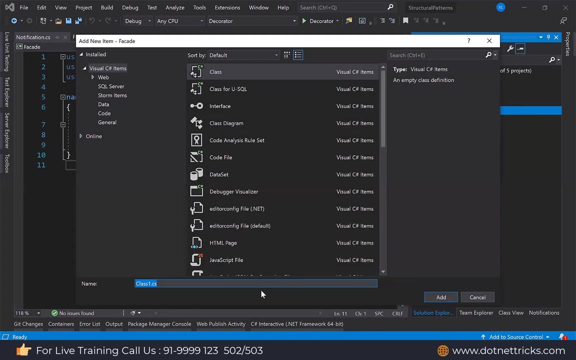 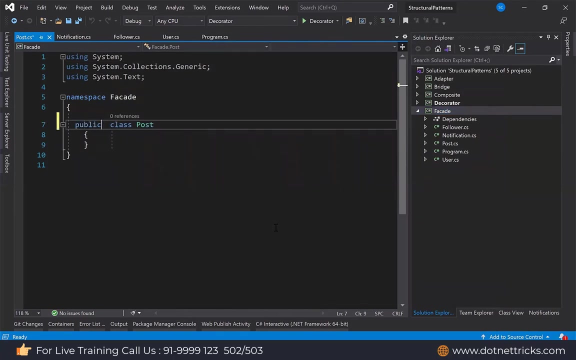 also. so let's say I'm adding a one more class for the follower and we will have one more class to send the notification. so we have been a class for managing the notification and we have been given class which is going to help us to post the message post. so it will post the text. 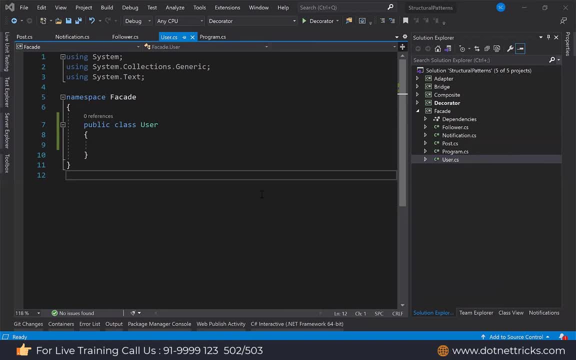 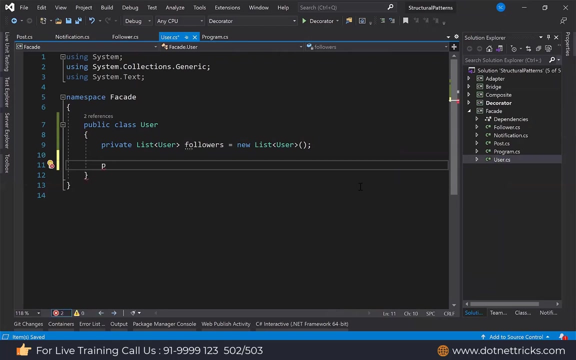 okay. so let's start with the user class here. so in the user class, i'm just going to make a list of followers, so private, i'm just going to make a list of followers for a user, how many followers we are having for user. so this is the user followers then what we have in common. so we have in common, let's say, user name. 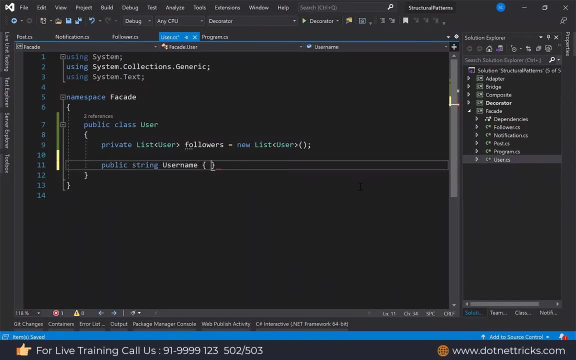 string. i'm. i'm keeping the class simple and short, so i'm adding here only one property: username get set. so through the username we can follow to others people as well and all the operation can be done. so here i'm having a method. let's say public boolean. there is a method follow, so here i will. 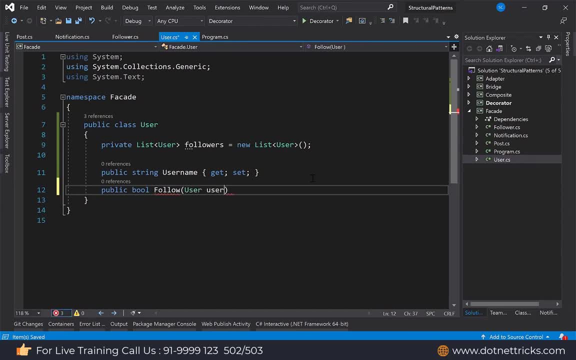 pass the user which to home i want to follow. so if you like, the code where you will store the information in the database, this user is the follower of this user. that code you write here. i'm keeping it simple. so code you have to write, i'm just returning here. true? so let's say we just store that information database now here. 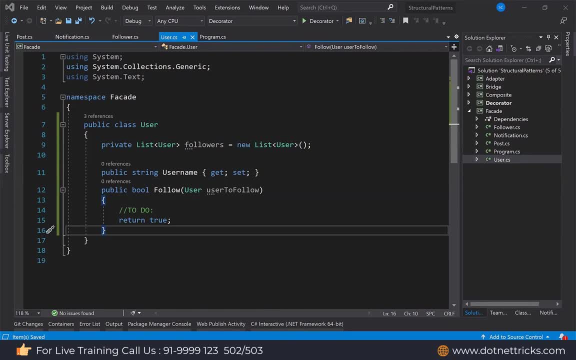 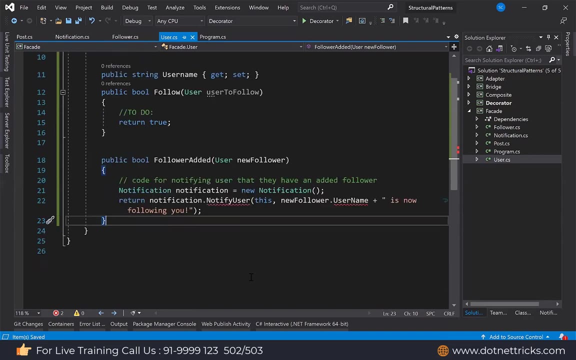 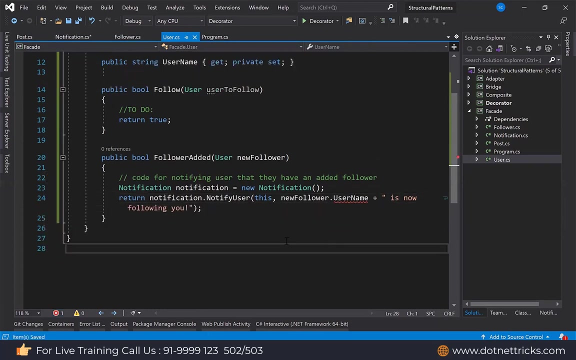 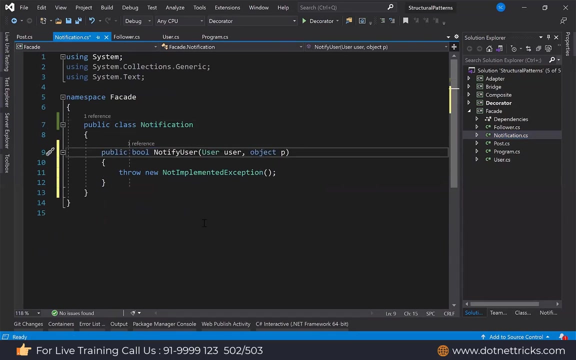 i'm adding another methods using that we will send the. so if this will be succeeded, so we need to notify. so here i'm having a method where i will add followers added and in the notification class i will add a method notified to the user. so this is my notification class where we will have a method notified to the user. 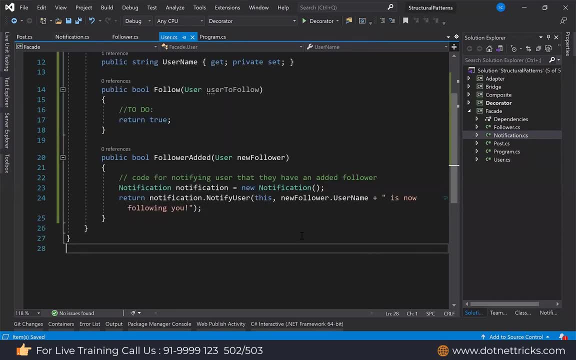 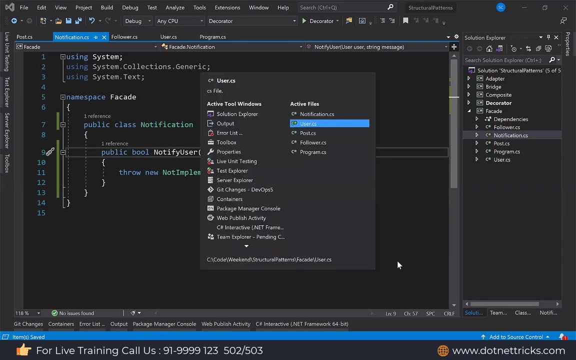 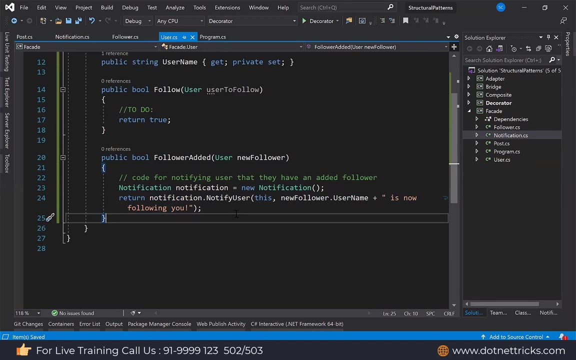 where? where i will pass the user and i will pass this message. what are the message you want to send to the user that can be sent through this? notify user. even the same thing we will get when we start following to a user on twitter, so that that user get the message. user abcd, start following to you. 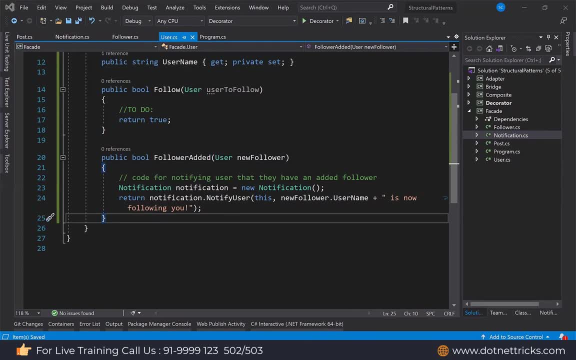 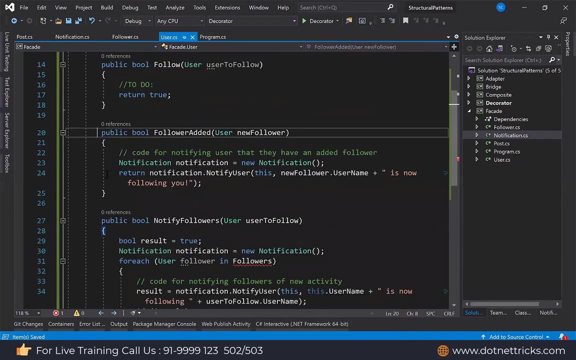 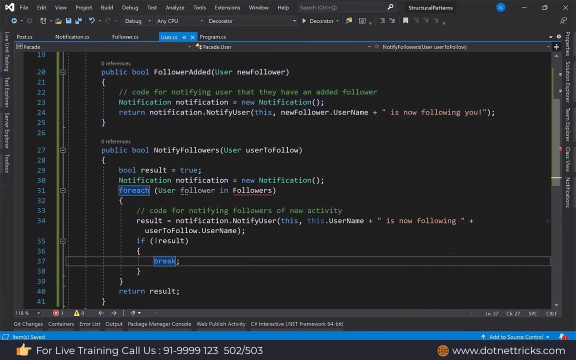 so same message i mentioned over there and we having here. so we having other materials. so notify to the followers. so the followers of that user also get notified. so notify to the followers. this is the information about the followers has been added. this is about like followers get notified. 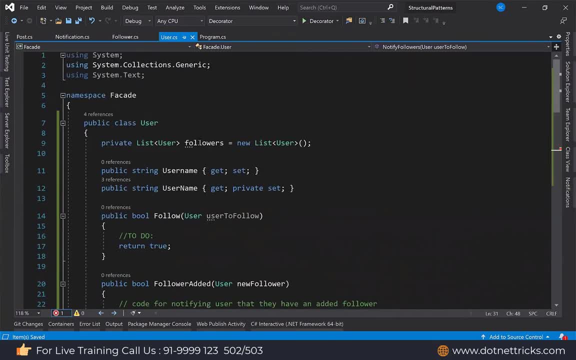 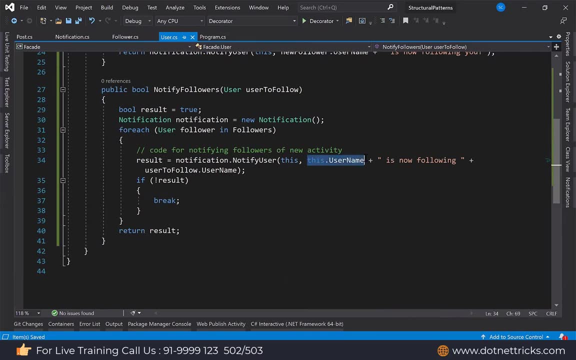 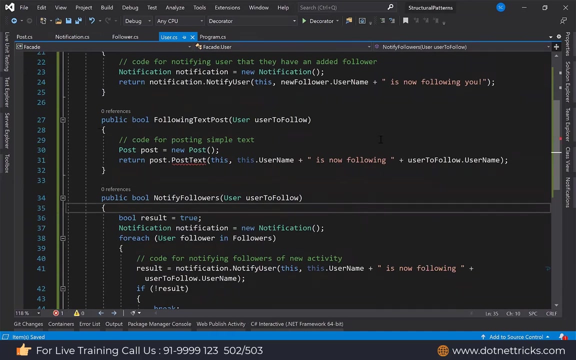 so let me mention the correct list over there: followers. so here we show us the message to the followers: user xyz now following to user abcd, so this will get notified to the followers. then we have been a method following text post, so we need to post this message to the public. 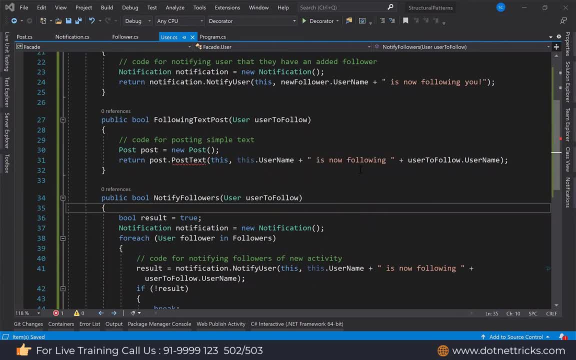 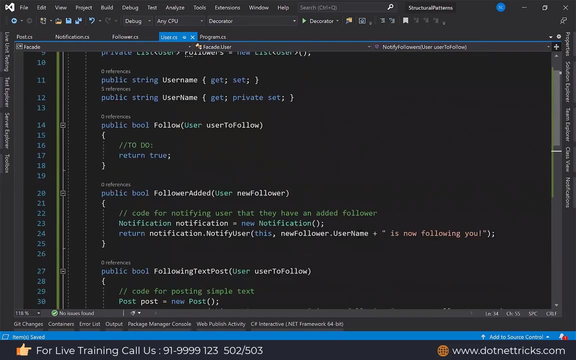 to a public activity for that particular user, like this user now started following to this one. so this is the public activity. so it's your just workflow. i'm just showing the way, let's say how- the simple workflow can be done here when you are going to follow the things. so in itself it's a complex things when it is coming to. 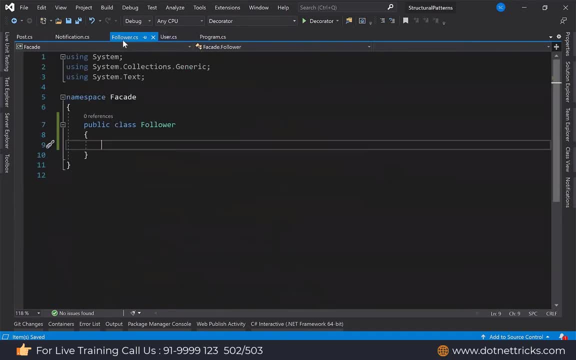 the system. i try to simplify it. now let's look at the notification class. so in the notification class i'm just having a simple console dot right line where i will write the message: console dot right line, that message. this way obviously you will save it somewhere and you will have some notification system behind the scene. 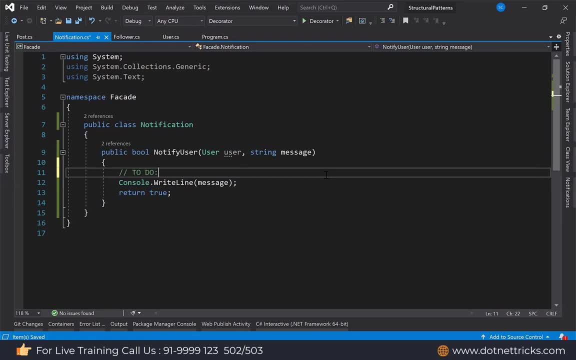 everyone. you can send the email also. okay, it's your implementation which you need to do over there. i'm just showing the simple message. so here you can send the email. you can send the asset, ms. it's your workflow. this is about the notification. we have done. 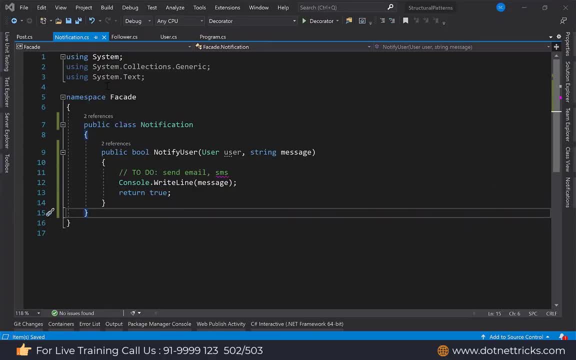 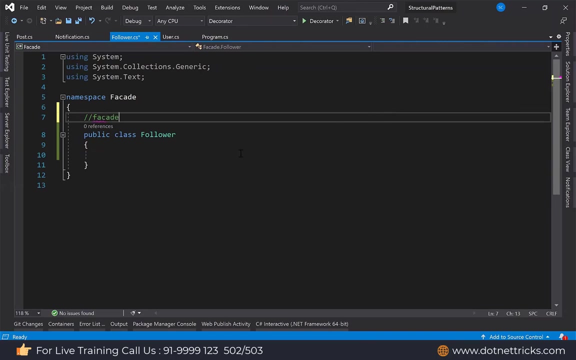 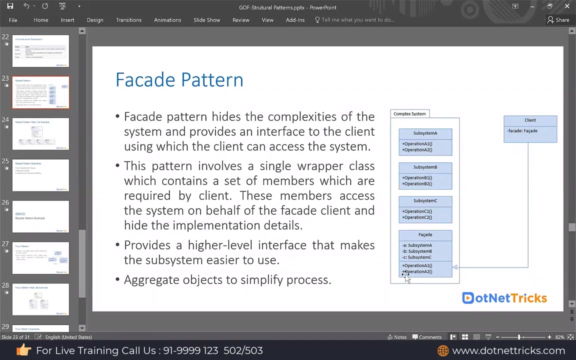 now let's come to the follower class. so in the follower class we will have a method follow. so actually this follower is acting as a facade. so what is happening here? if you look at the pic here, there would be this facade. that facade will have the information about system a, system b, system c and the client will expose to the 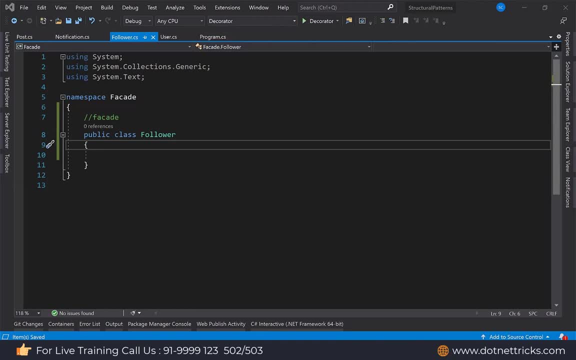 this facade. so at the followers label and the, that code will be right here. so here i'm just going to write a method to follow the people public boolean and follow is a method over here. then i need to pass the user follower, who is the follower and who is following. 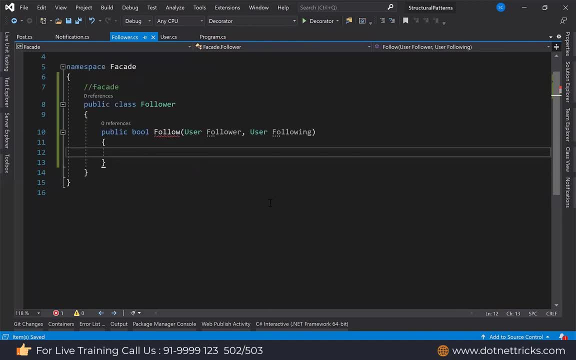 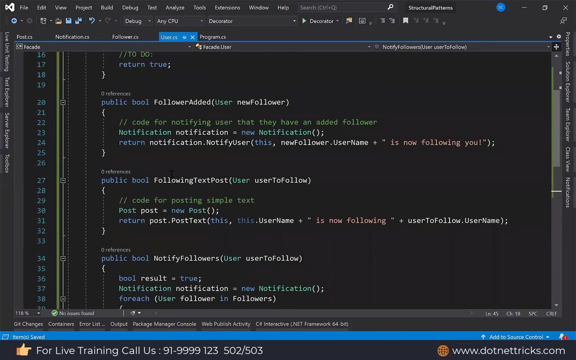 this is the one. so two parameter i will pass here: follower and following. then here let's say: we having a result, now using this follower, we will do the operation. so here we will have here, let's say, add the user as follower, so that code we already written in the user class. so we are being a 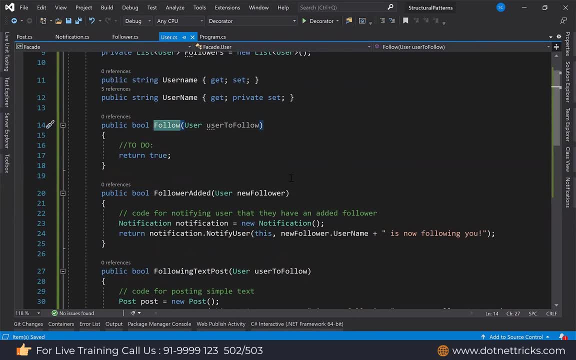 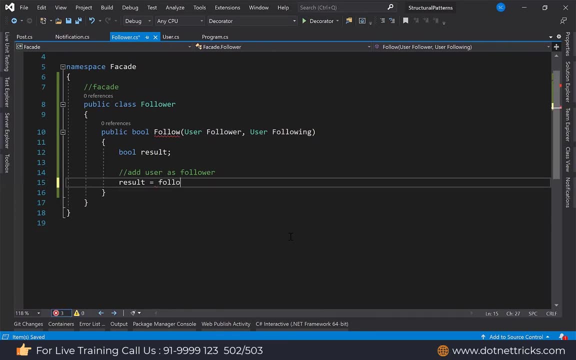 method in the user class follow. so this method i will call here, so it would be here: result equal to follower, then follow and to which user you are willing to follow. i'm going to follow this one. following in this way. if result is succeeded, then fine. if it is false, then 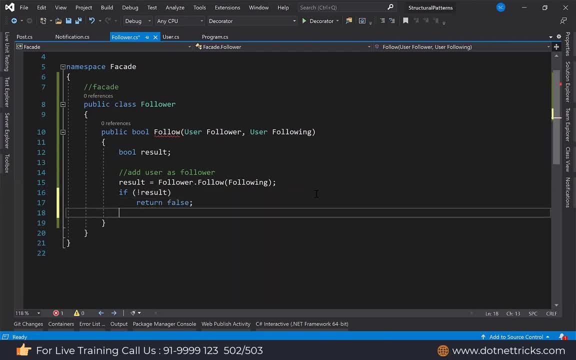 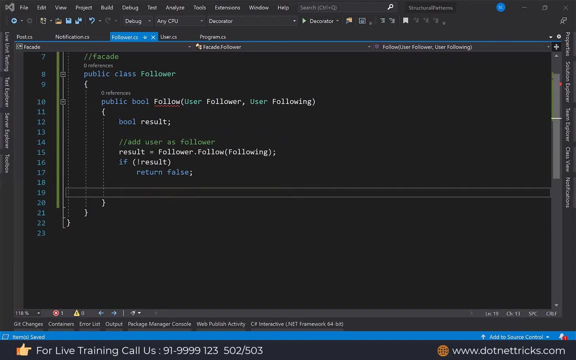 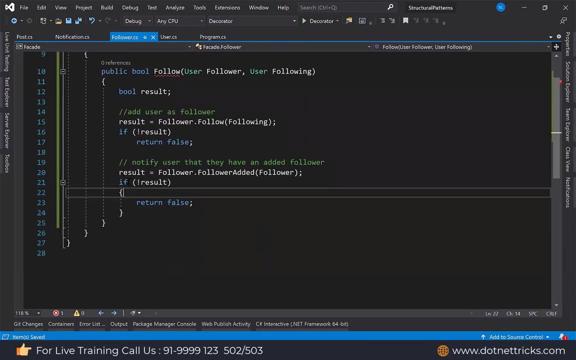 return false here means something is not working. fine. same thing. i need to add here another method: followers added, so add the followers to the database over there. so this is the same thing. i'm just using here written false. now post the message. who is falling to which one? this is the one now notified to all users. see, i'm. 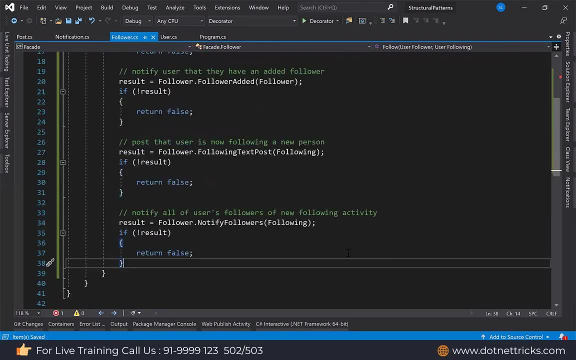 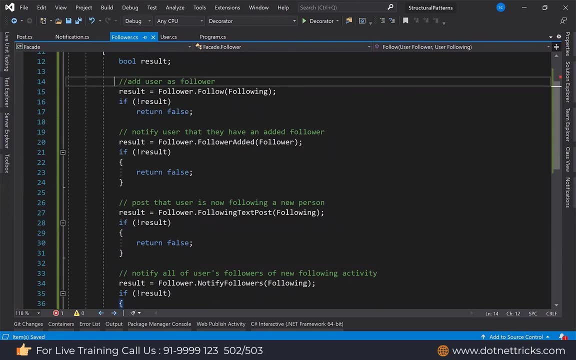 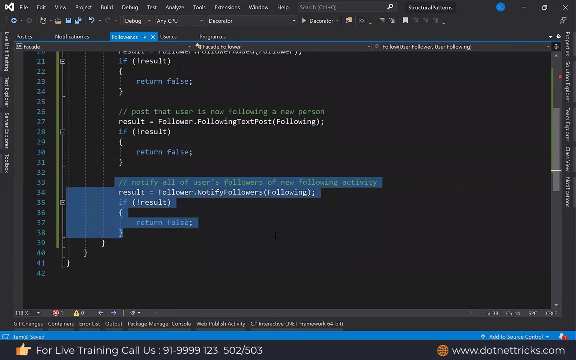 way. this is the way. so this is the way how we just simple, we just creating a process in one. in the first step, we are just going to follow. in the next step, we are deciding the followers, and the next step, we are posting the information. in the next step, we are just notified to all others. followers like this person start falling. 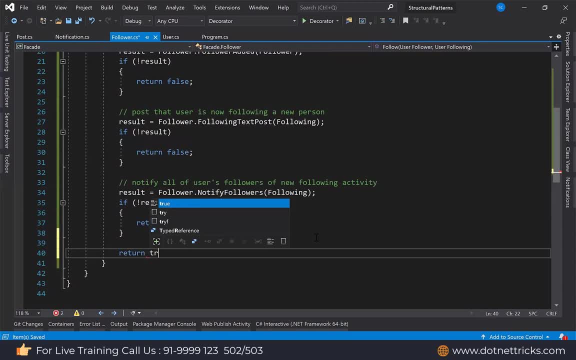 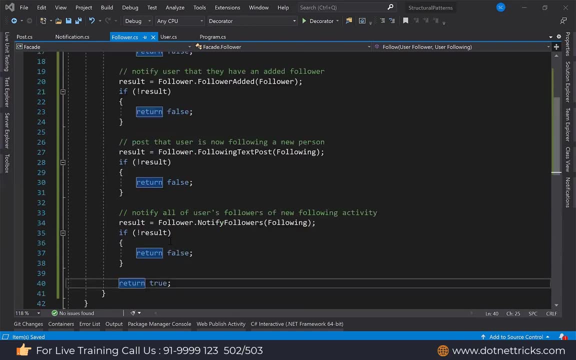 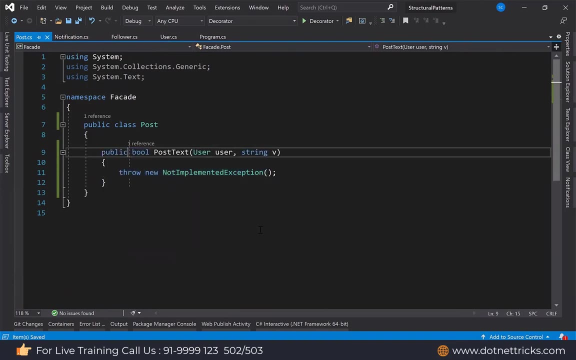 to this person and finally written true, if everything is fine. so now in the post class where we have not written the any okay implementation. let me implement what the message you are going to post over there, so there would be your own code which you will implement. i'm just writing here a simple console dot right line. 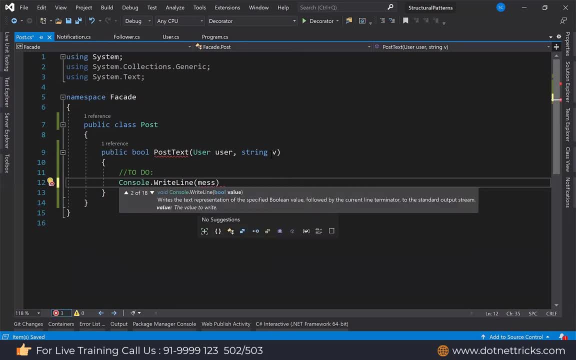 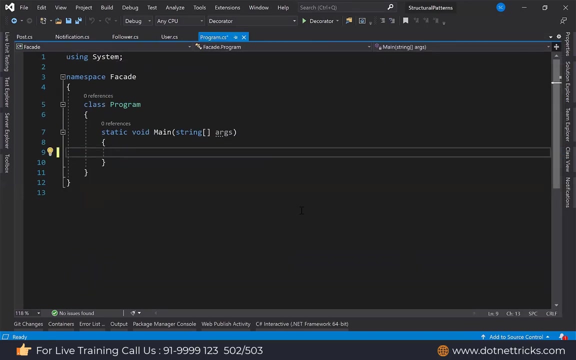 method where i'm just going to use the message message and finally written true this way. so now here comes to the program class. so so first of all we need a user which will follow to the another user. so here we. we don't have anything which is coming dynamically from the database. 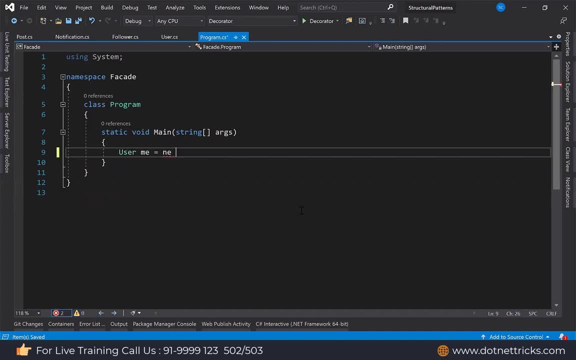 so what i will do here. i will create a user- let's say it is me, so it is me. and let's say my username is here: username equal to pro shalendra. this is my username at twitter. let's say to which i'm willing to follow. i'm willing to follow user i want. 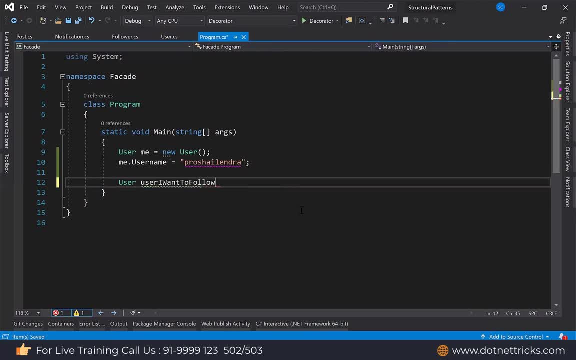 to follow. let's say, this user will come from the database, but here we don't have anything dynamic. so i'm creating a user for myself and a user which i want to follow. user which i want to follow- having a username dot net tricks- is the user which i want to follow. so now here i'm just. 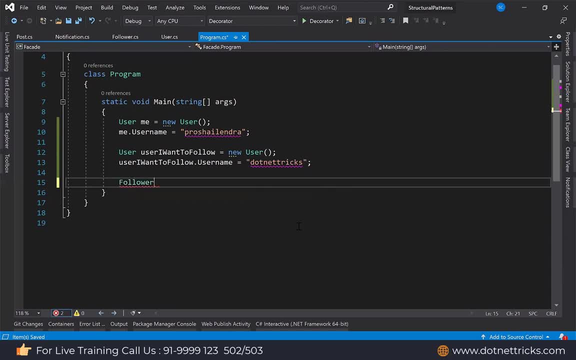 going to create here a follower like facade, because i said here i need a facade object, same i'm using here now choosing the facade. i can access it here. follower equal to new follower. now let me check follower if following the thing successfully, to which one me and user. 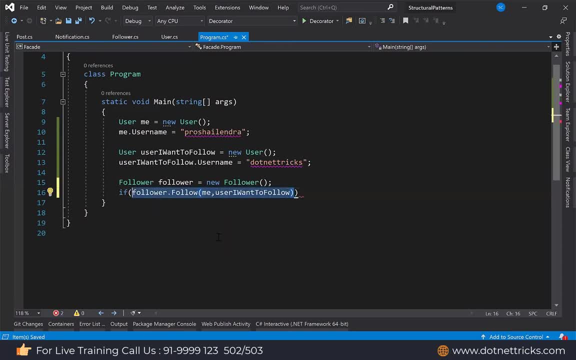 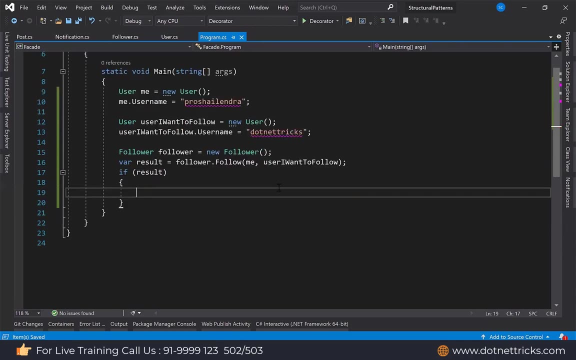 which i want to follow. let me simplify this code here. where a result? this way: if a result is true, they should write the message you have successfully followed to that user. this way, if there's an issue while following the user, so i can show a message. sorry, something went. 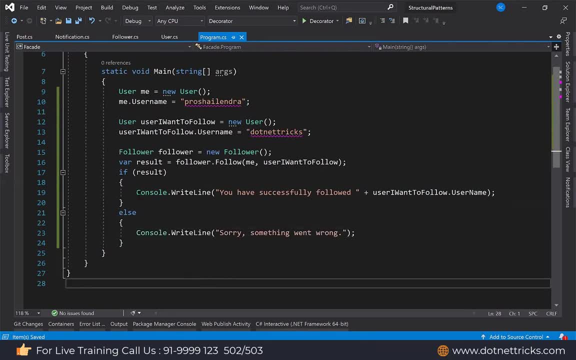 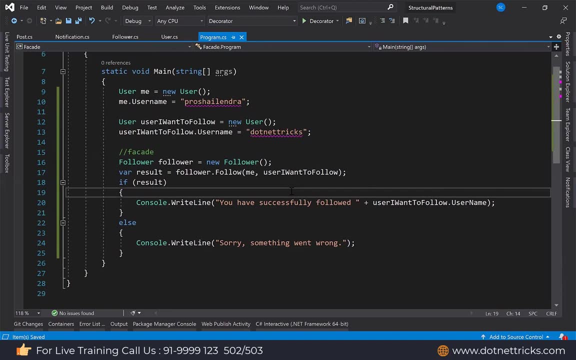 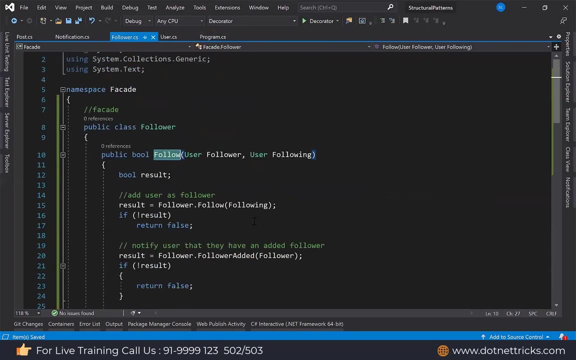 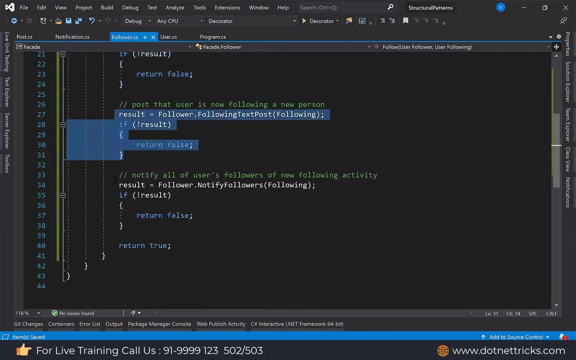 wrong this way. so this is my facade through which all the things we are implementing. so, if you will look at in this follow method, the process is complex. it's not simple. first we are using this one, then we are doing this one, then we are doing this one, then we are doing this one. but everything is hidden from this. 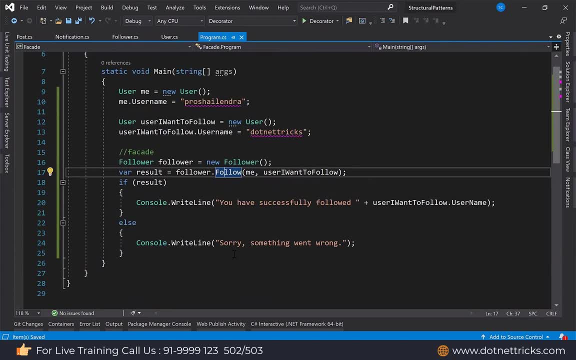 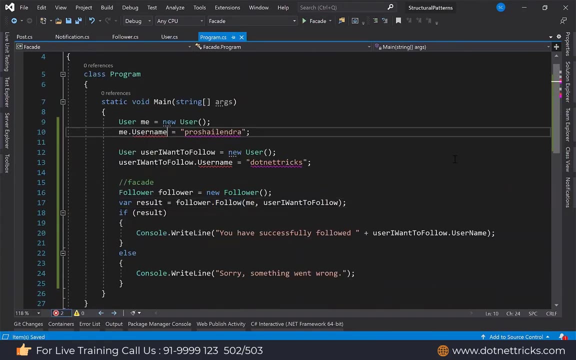 before the hello. it is only calling the one method and internally it is happy it is handling all the things. so let's run the code here for the facade. so here i'm just going to Run the code for the facade now. let's run it. ok, now in the program file it should be this username: 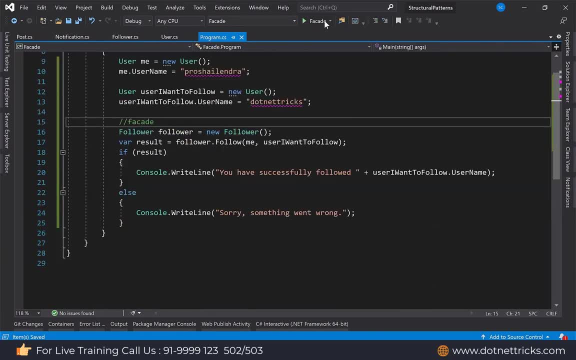 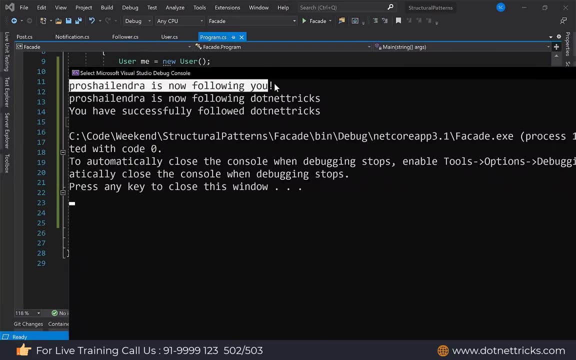 so there was an error while setting the value. now let's turn it open So you can see here. the pro challenger is now following you. Pro challenger is following to dotnetrix. You have successfully followed the dotnetrix. So, basically, these are the notification we received. 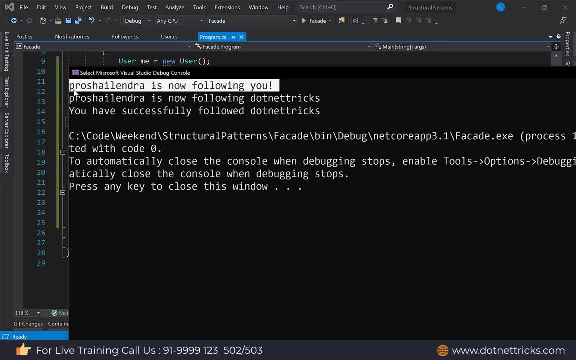 So this is the notification the person will get to whom you are following And this is the message you will get here. like that person, friend, will get this message And this is the message you will get. You have successfully followed to the dotnetrix. 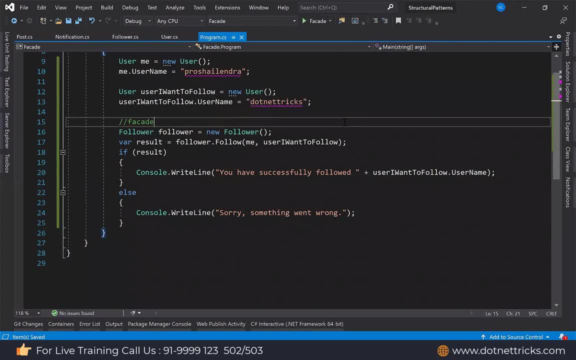 Got it. So this is the way how the facade can be implemented. There can be so many other examples which can be used. where the facade can be used, I'm sure the similar thing you might be using somewhere, but you don't know the pattern. 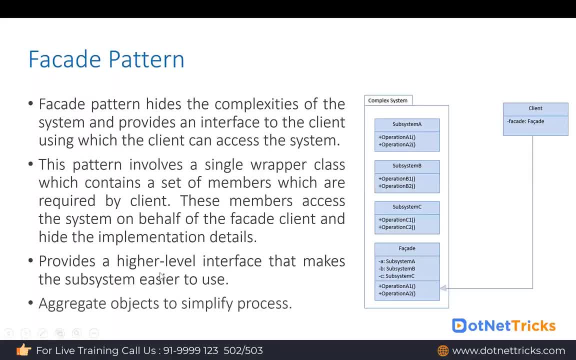 name, Isn't it? So facade is a commonly used pattern. 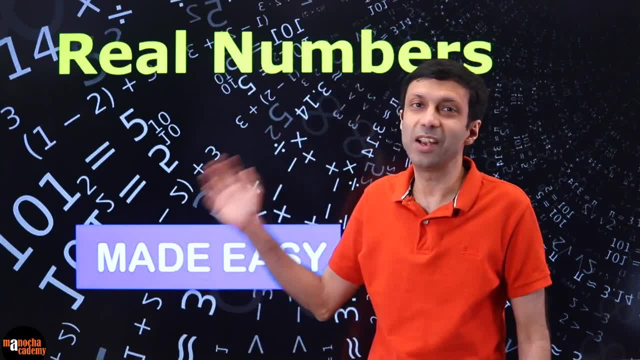 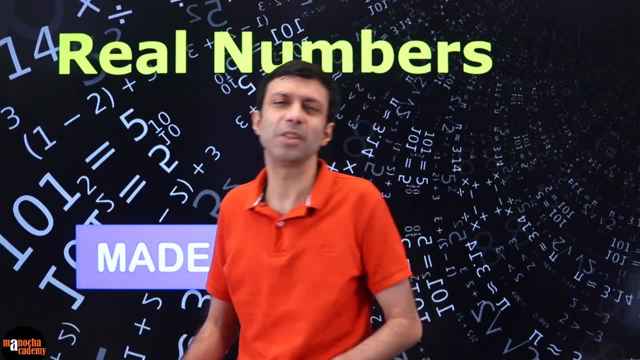 Hi guys, welcome to this class where I'm going to make real numbers really easy for you. This is also called number system in some of the textbooks. So whether you call it real numbers, number systems, let's get these number concepts crystal clear. Keep your pen and paper ready. 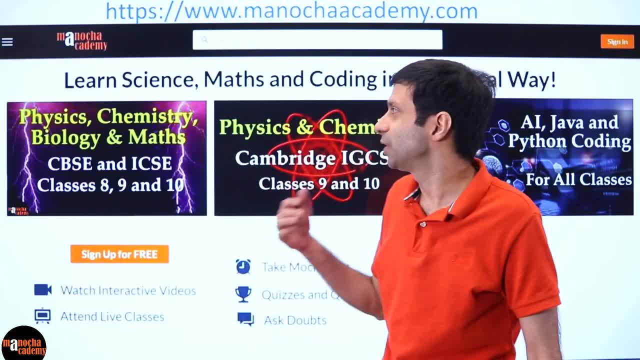 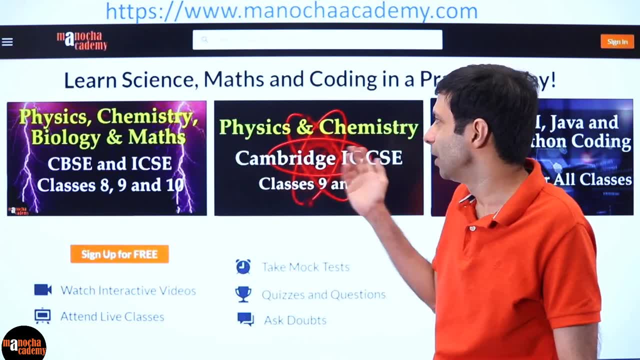 and let's begin. Before we get started, I just want to say: do check out the other courses on our website, if you haven't done so already. We have physics, chemistry, biology and maths for CBSE, ICSE. We also have the Cambridge IGCSE International Board And guys, check out our AI. 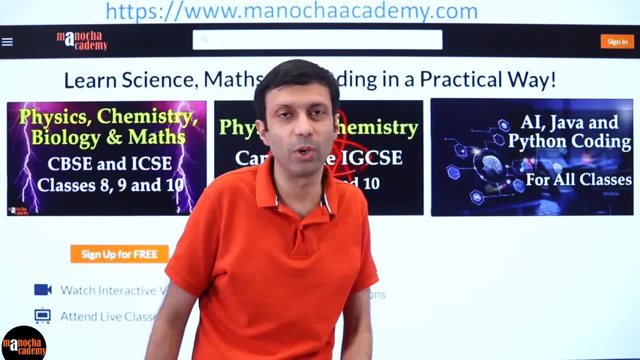 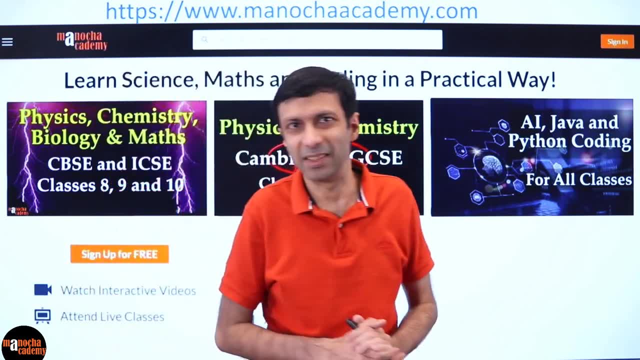 our new course on artificial intelligence. We have Java and Python coding for all classes, So do share it with your friends and make sure you have also subscribed to our YouTube channel. With that let's begin. We're using numbers all the time in our daily lives. right Like let's. 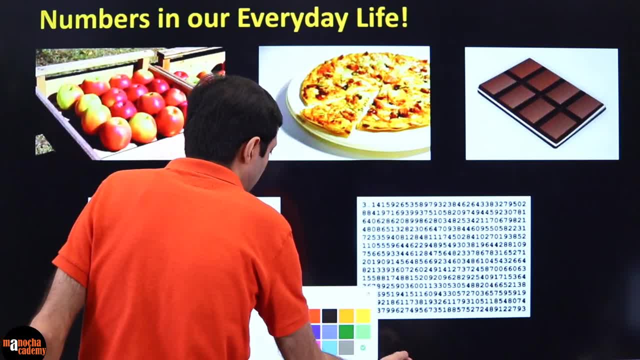 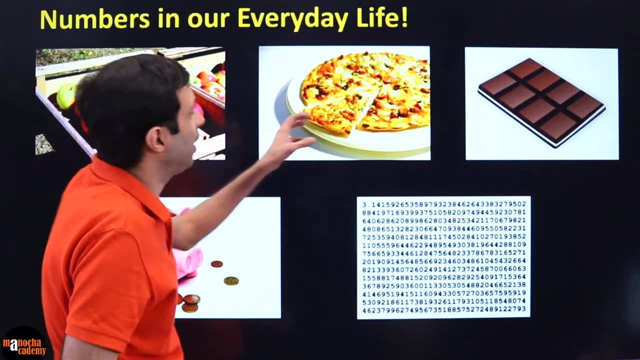 say, our mother tells us get some, you know a dozen apples. or in this picture, I think there's 16 apples here. So you can see in this box that's the number. So let's get some apples- Number 16.. Oh, I'm feeling hungry seeing this pizza. If I eat this pizza slice, how much of? 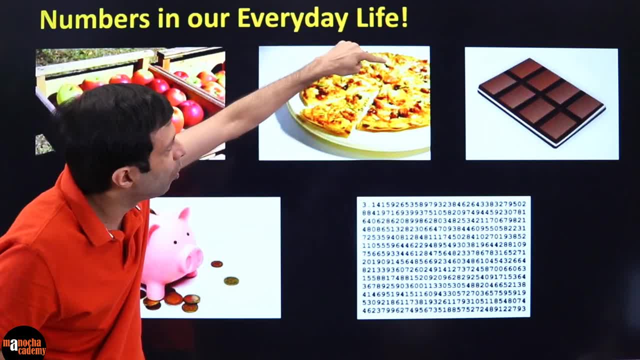 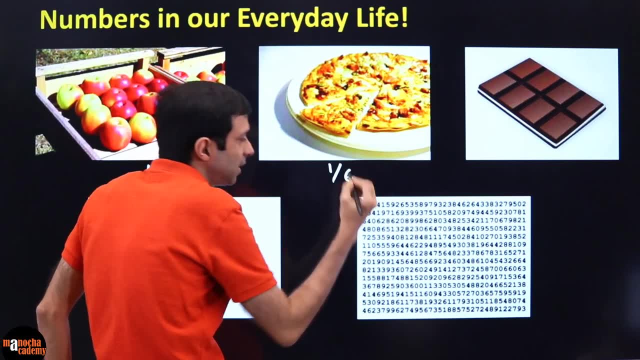 the pizza I've eaten. Can you see? there's 1,, 2,, 3,, 4,, 5,, let's say, 6 pieces here. If you eat one slice you can't say you've eaten one pizza. you have eaten 1 by 6 of the pizza. right Fractions.